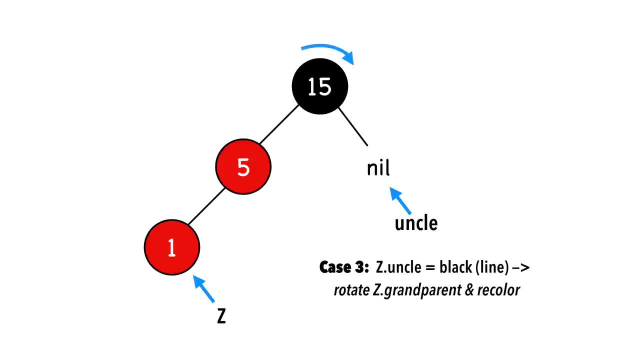 We rotate Z's grandparent 15, in the opposite direction of 1.. Finally, we recolor the parent and the grandparent. We're back to a balanced red-black tree. Pretty simple so far. Let's move to a large tree and see how we use each case sequentially to fix violations. 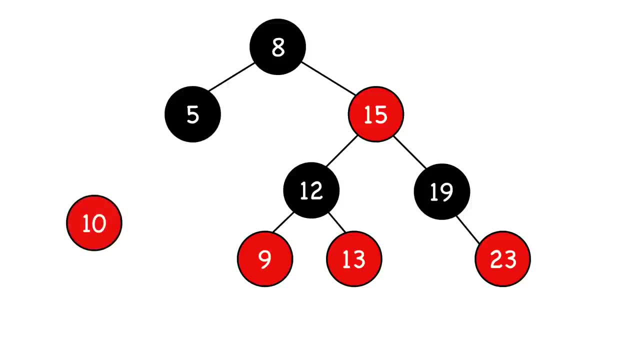 We'll start by inserting 10.. Then we'll add 10 to our tree, coloring it red. If this was just a binary tree, 10 is in the correct spot, But since this is a red-black tree, we need to fix the violation. 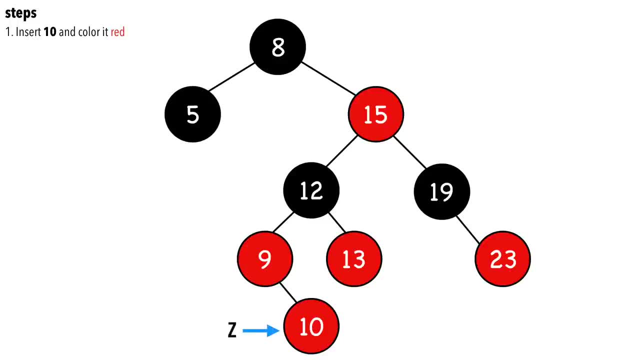 10 is our Z and Z's uncle 13, is red. This is case 1, so we'll recolor Z's parent, grandparent and uncle. The tree is looking better, but notice that we just moved the violation up the tree, as 12 and 15 are both now red. 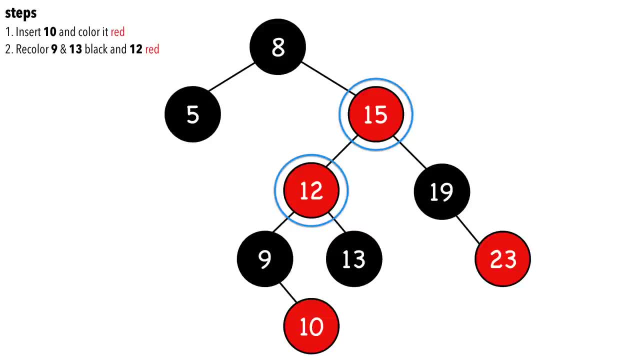 We must keep fixing the tree until all red-black tree properties are met. So let's apply our strategy on this new violation. As our violation moves to the top, we move Z as well, setting the pointer to the violating node In this situation. it's 12.. 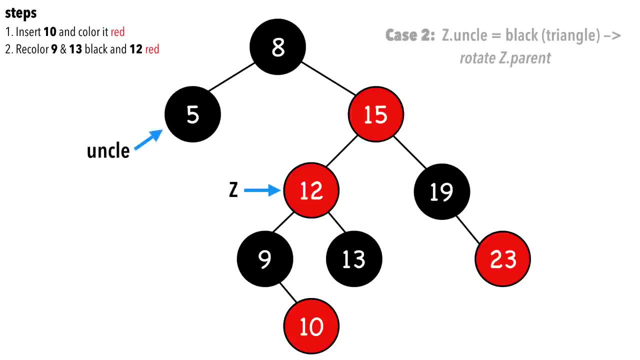 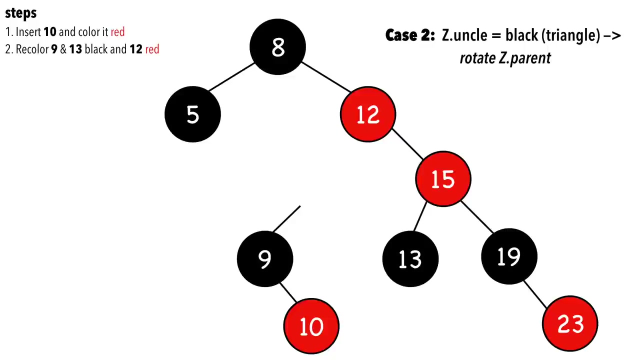 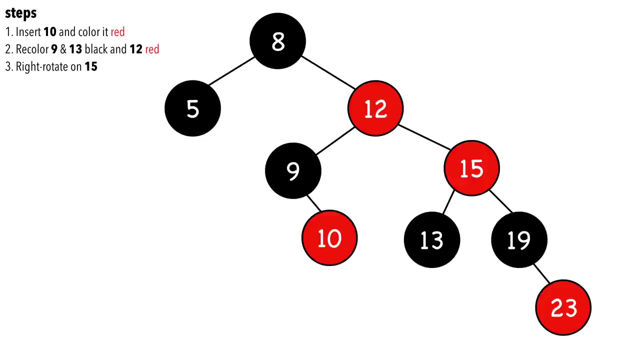 This looks like case 2, as Z's uncle is black and a triangle is formed, We do a right rotation on Z's parent, which is in the opposite direction as Z Almost there. We'll set Z to 15 as it is the violating node this time. 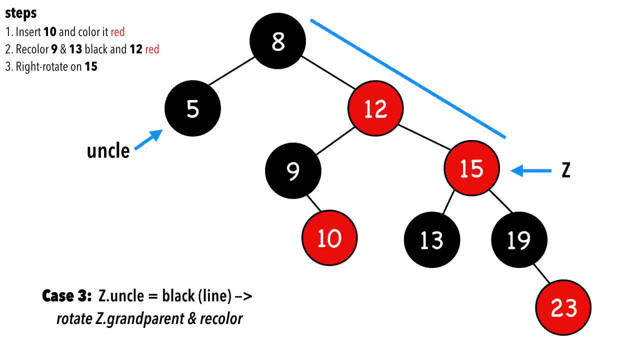 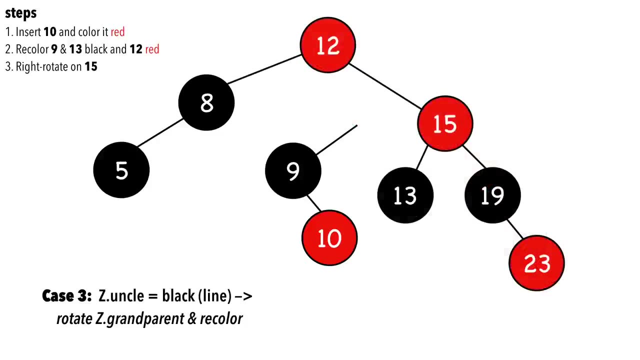 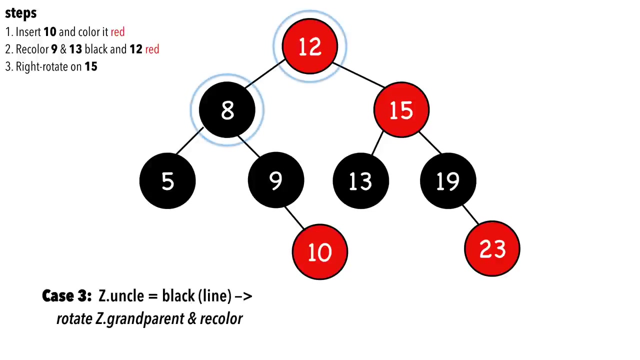 This looks like Case 3, because a line is formed. We do a left rotation on 8.. Finally, we recolor 8 and 12, Z's original parent and grandparent. The tree is rebalanced and free of any violations.